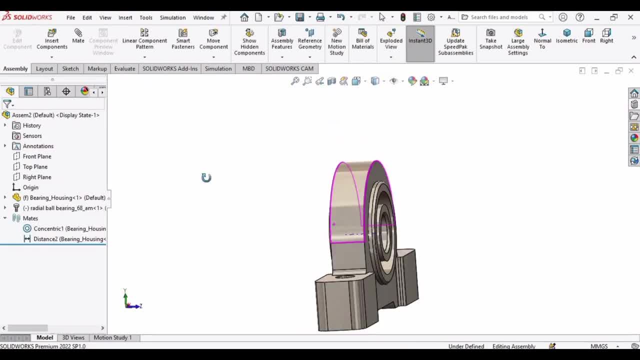 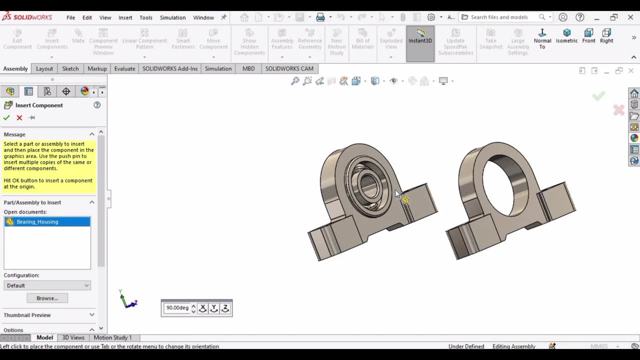 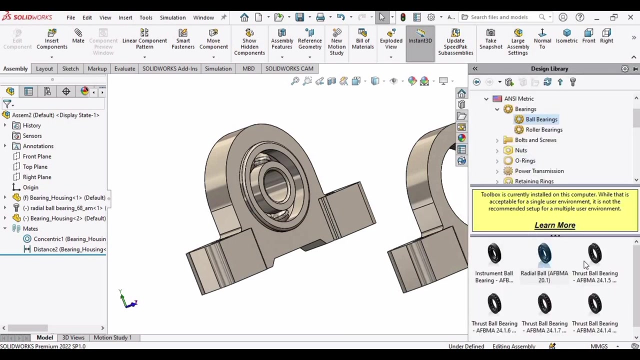 And now press enter. Here you can see the bearing is aligned with the housing. And now let's rotate it. And here you can see the bearing is working fine in the housing. So insert another bearing housing In this environment window. And now let's insert the same ball bearing again. For that go to design library and insert this. 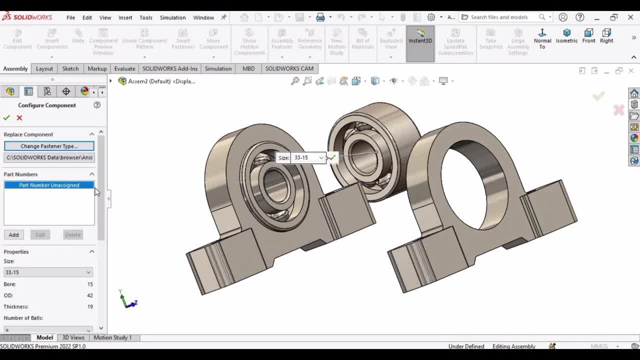 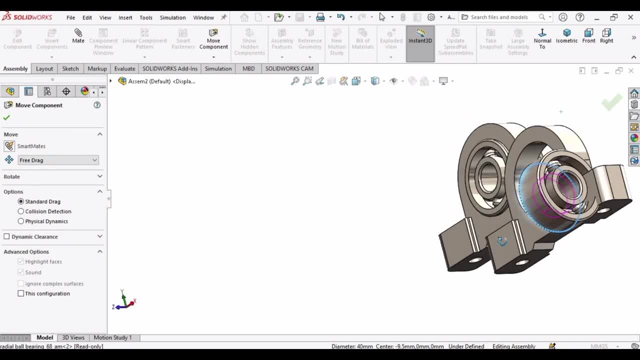 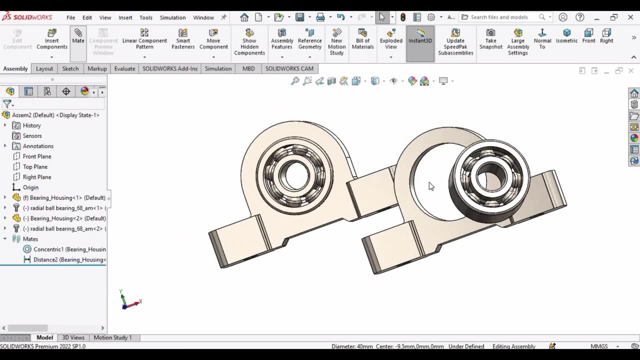 same radial ball bearing. here, in this environment window, We do not need to specify any parameters, because we have specified earlier. So now let's adjust it, Move and rotate. And now click on this mate option. Select the inner surface of the bearing housing and outer surface of the bearing. 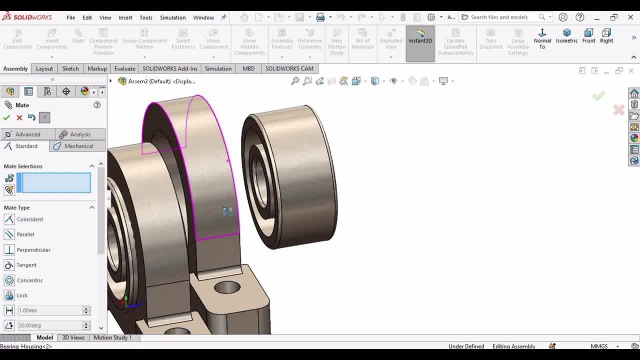 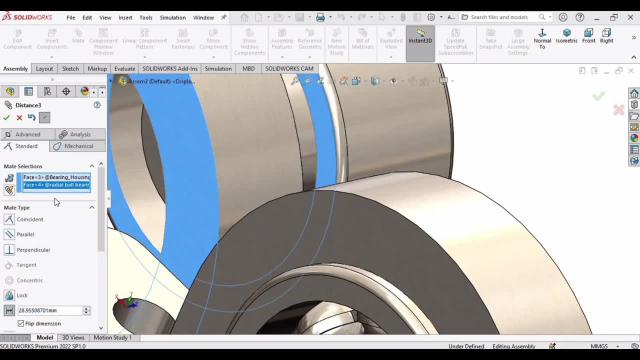 And similarly, just select the side of this bearing housing and the side of bearing, And we need to specify some distance here. Specify 2.5 here. Okay, so it's not working. So cross the window again and select these two walls again and specify the inner surface of the bearing housing. 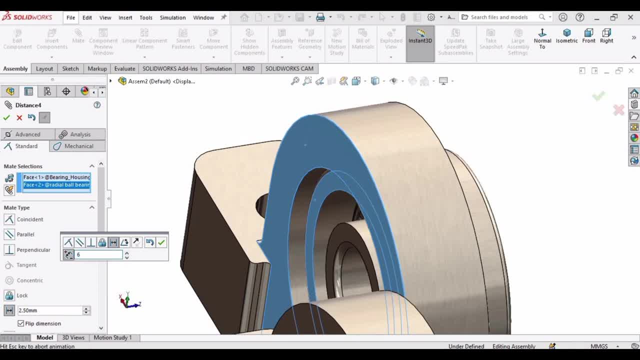 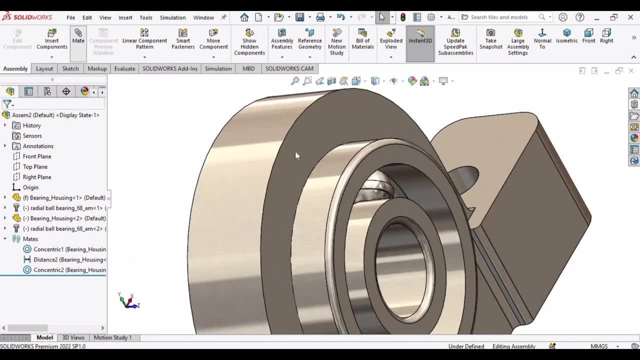 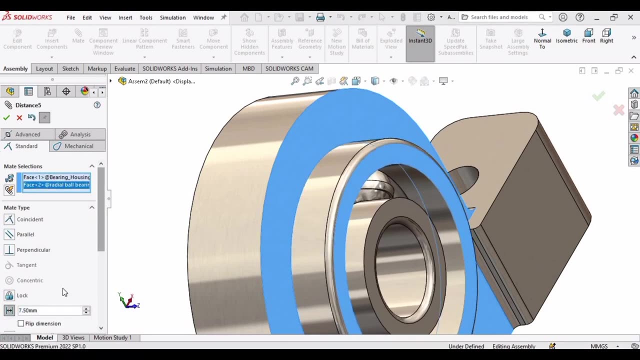 And specify the distance as 2.5. But I think it's not going to work on this side. So move to the other side of this housing, Select mate. Select this side of the bearing housing and this side of the bearing And now specify 2.5. And now it's working properly. 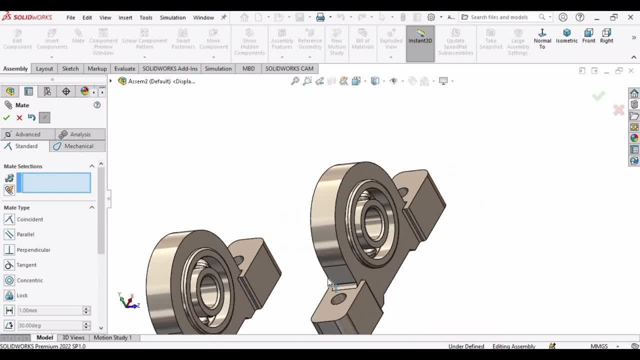 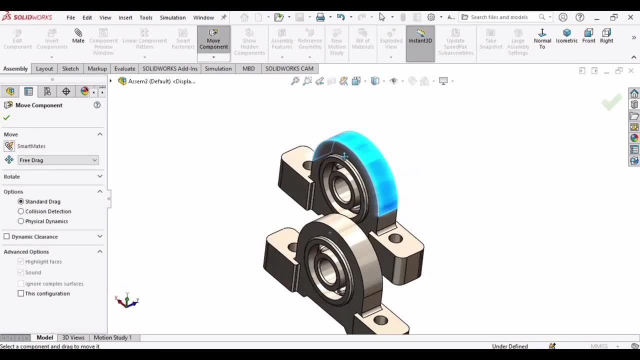 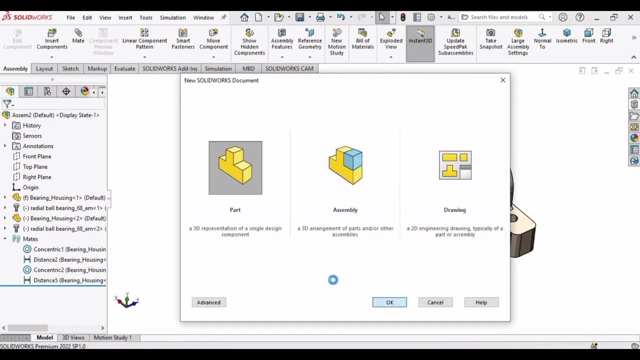 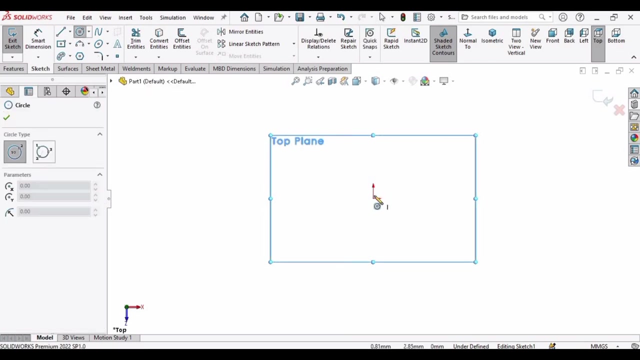 And now both housings and bearings are ready. Now we need to set the distance between them. so move this bearing housing here and now. we need a share for that. open a new file. open a new part file. specify the background as plain white and make a sketch on top plane. make a. 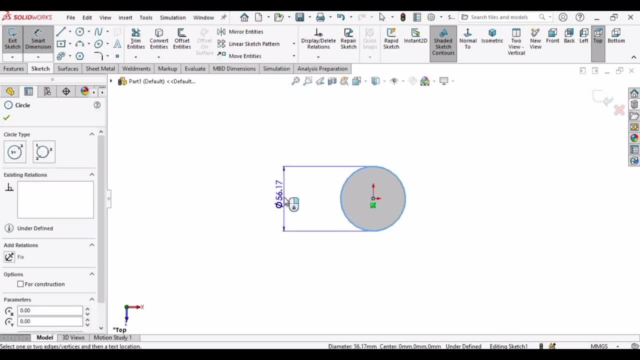 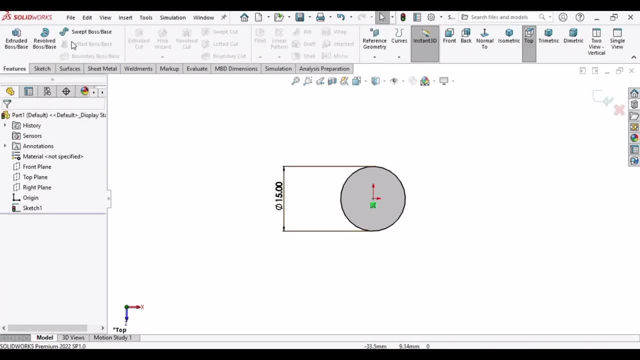 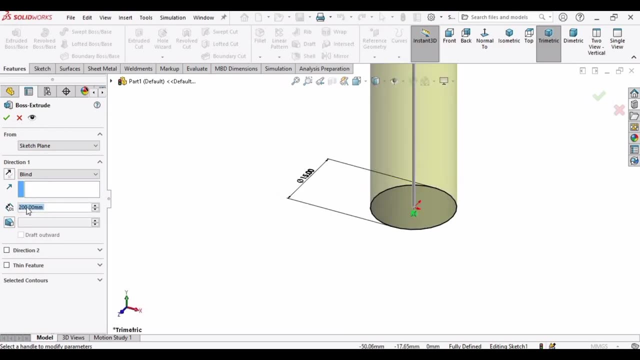 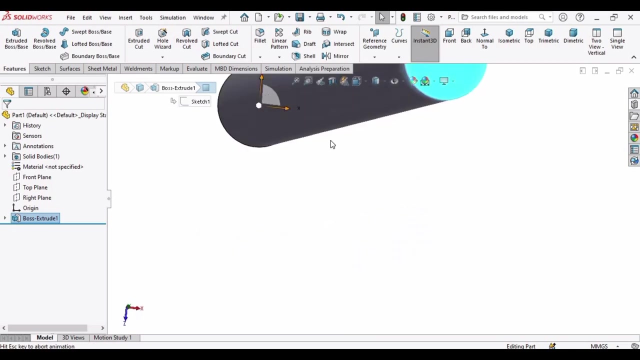 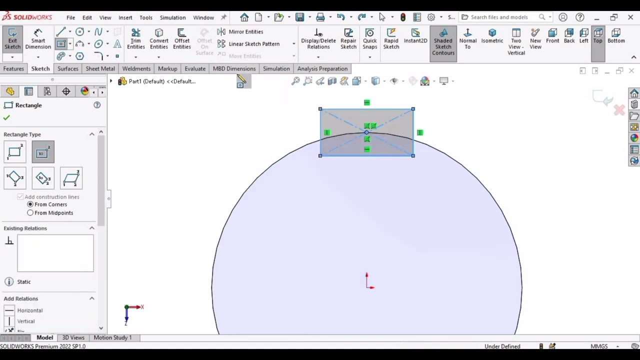 circle here at this origin. specify the diameter as 15 millimeter and then simply go to feature. select extruded boss base and simply extrude it up to 200 mm. click OK and select this surface of the shaft. click on sketch and make a center rectangle here. now specify the dimensions. 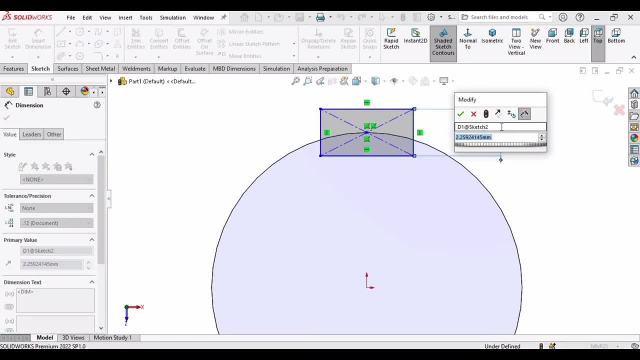 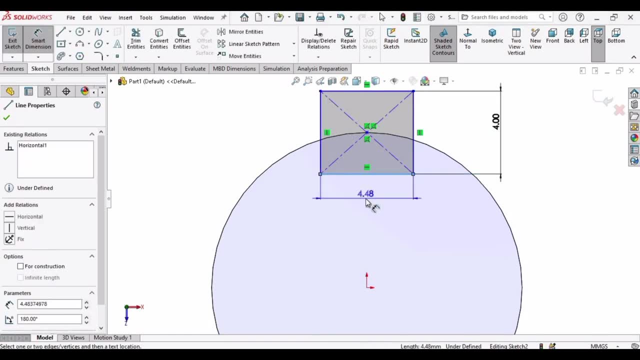 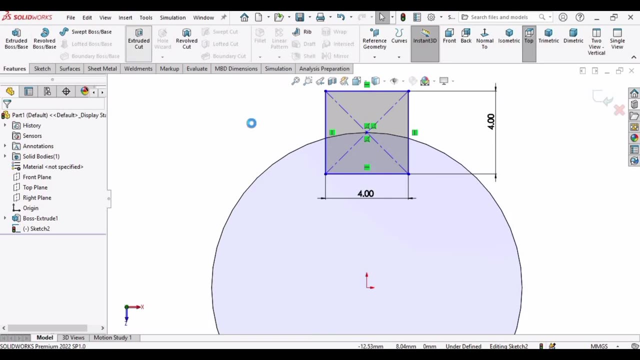 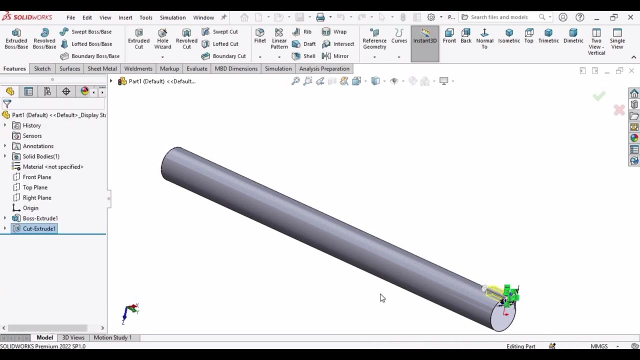 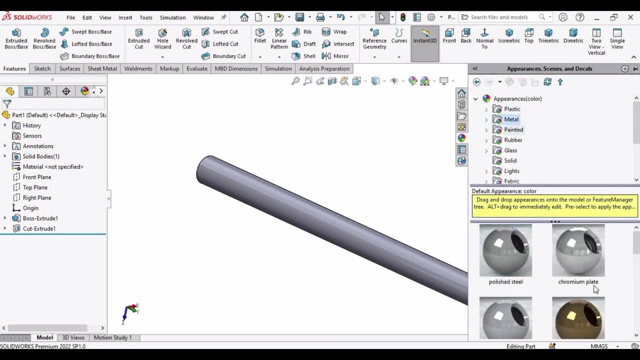 specify each side. as for specify here as 4, click enter and simply specify the dimension of this side as 4, then click enter and now go to features, select extruded cut this time, and here we need to specify 10 and then click enter. so specify some material to this. in metal, you can specify any material to this. 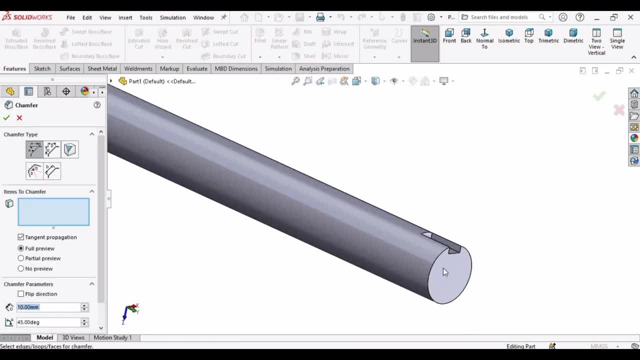 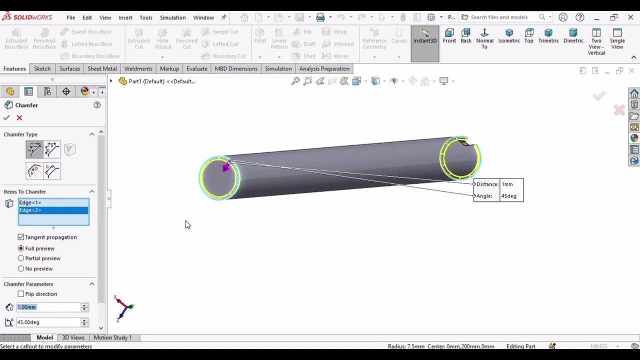 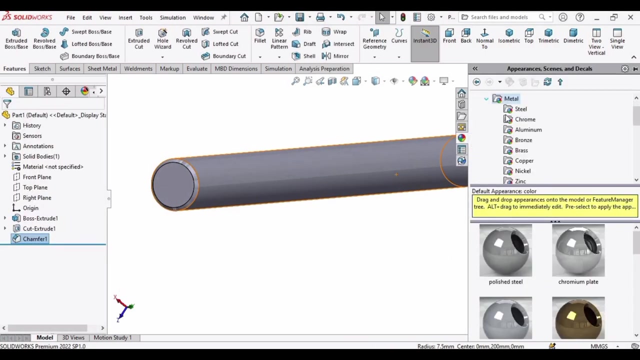 so and now make a chamfer here, select this edge, specify here too, and then select the other edge of this shaft- this one, I think one mm is fine for the chamfer- and then click OK. now here I am specifying some different appearance, okay, so now save this. 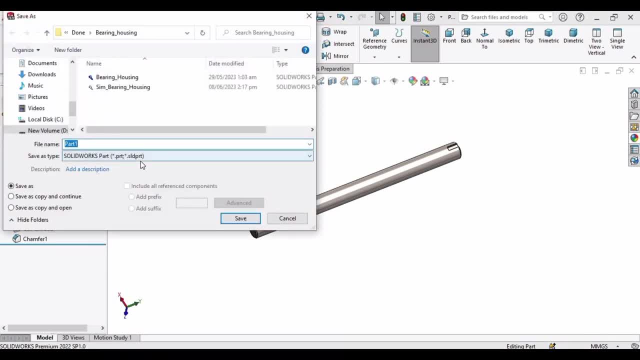 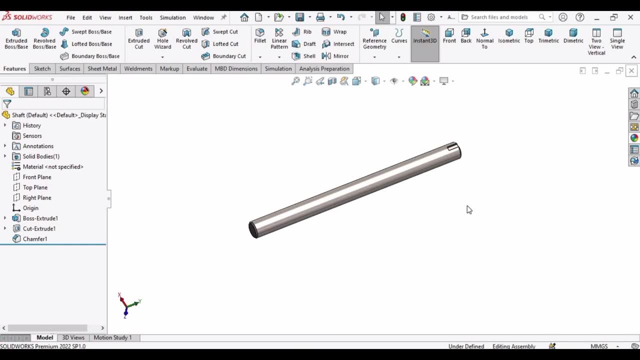 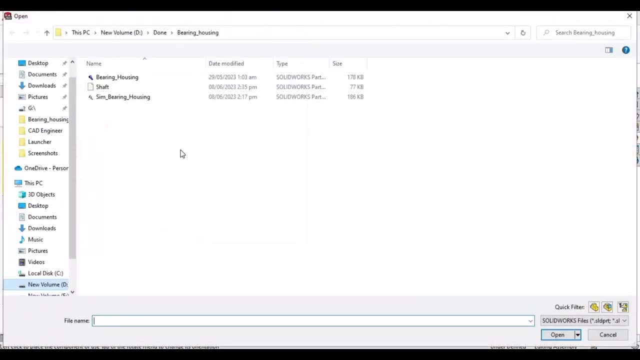 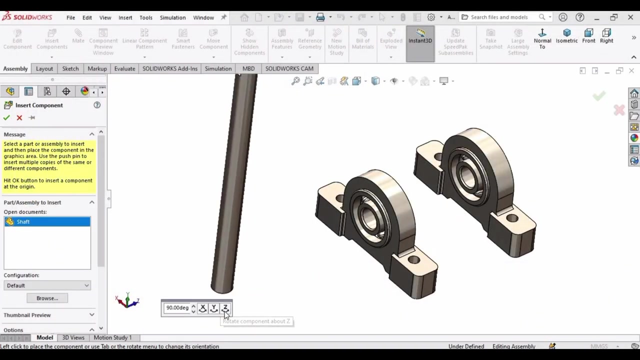 file as shaft, press ctrl s and save this file as shaft and then close this file and import the same file by clicking here in insert component, select shaft, click on open and here we we can change the orientation. click on y axis. now it's fine, so click here in this environment window, and now we have to align these two. 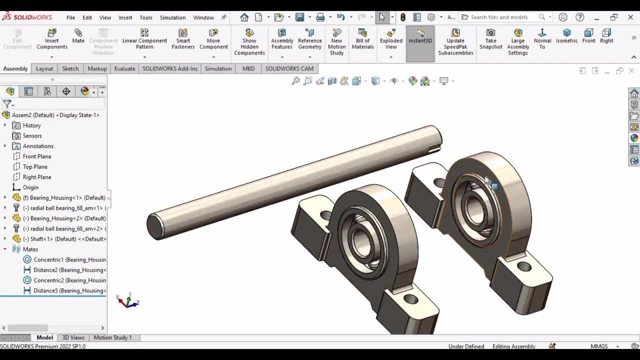 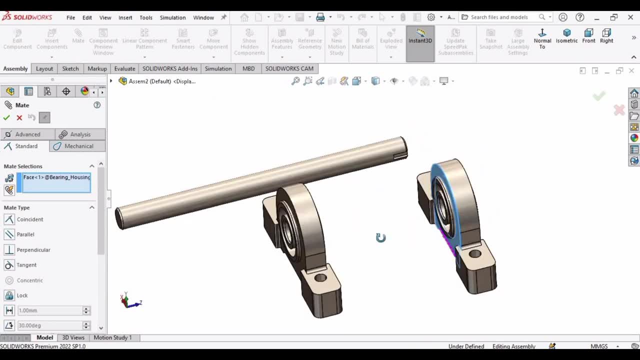 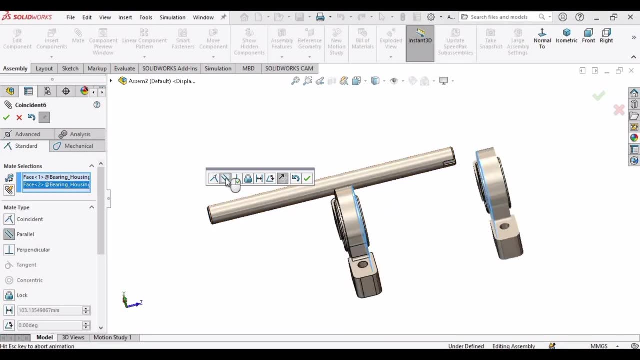 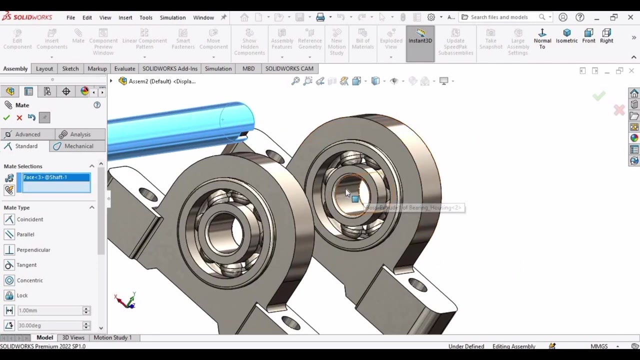 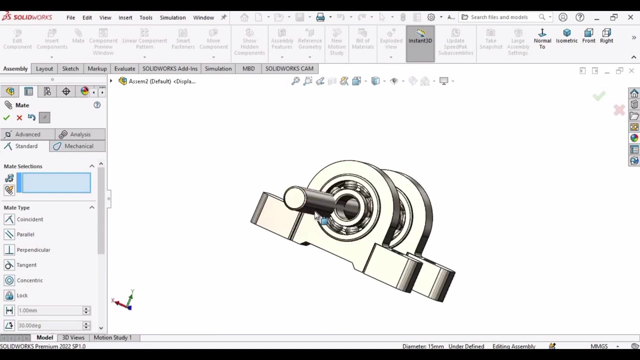 bearing housing first. so select this surface, click on mate and then select the other surface, the surface of the other bearing housing, and now we have to select this option parallel. okay, and now select the shaft again and the bore of the bearing. click OK and now select the shaft again and the bore of the other.